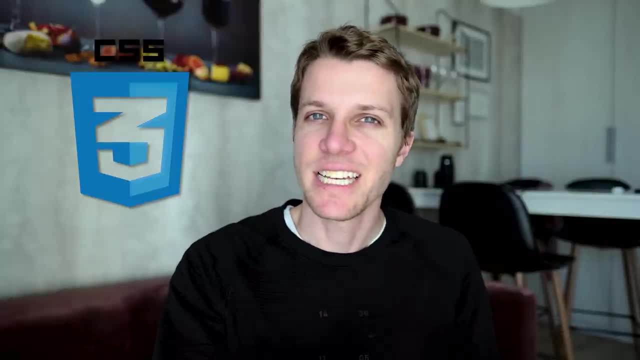 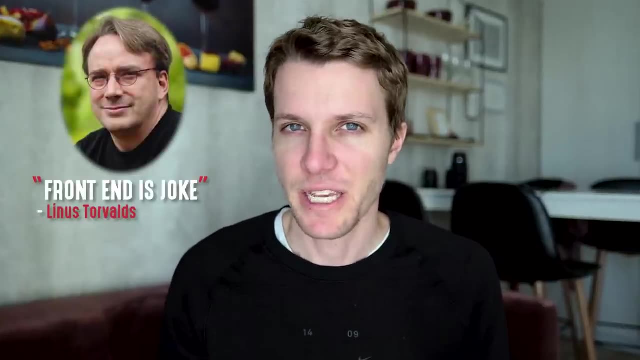 why, even though they look like code, you'll hear people say that css and html are not real programming languages. So it's not because they're back-end elitists, At least not in most cases. Anyway, programming and not coding skills are what most of the biggest tech companies test. 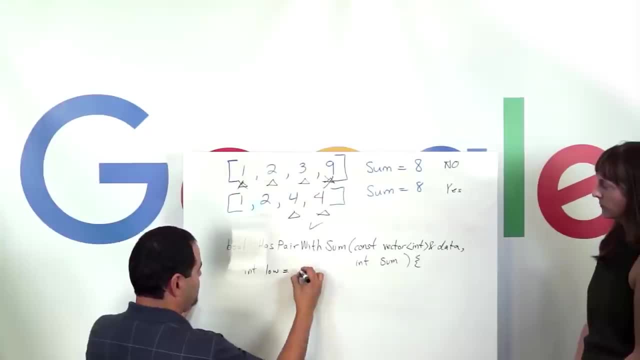 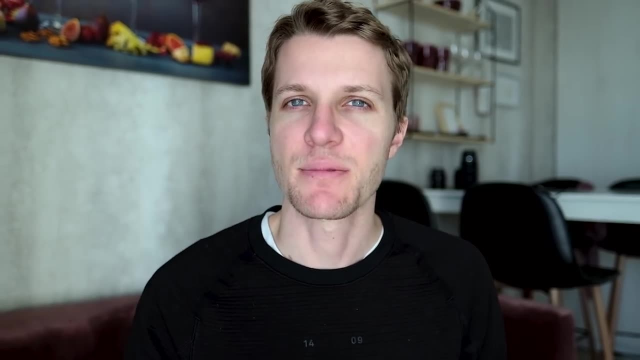 for, and it's why they let you take your interview a lot of the time in any language that you want. This is why these interviews are often done on a whiteboard with something called pseudocode, where you're just writing out steps in plain english rather than specific coding syntax. Now one final. 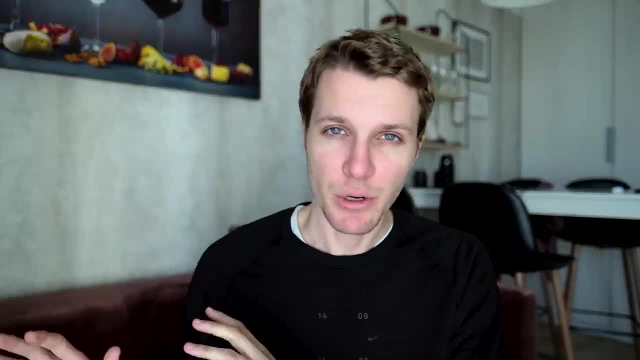 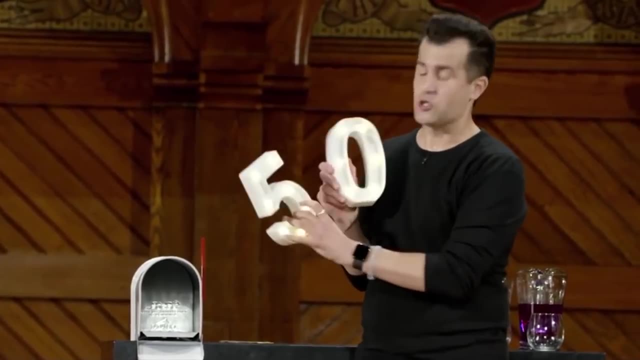 example, there's a course that focuses purely on programming and not coding, and that's Harvard's cs50.com. A lot of people are surprised when the first week in homework are not even in a real programming language. it's just some kid's programming language called scratch. Then from there the course quickly. 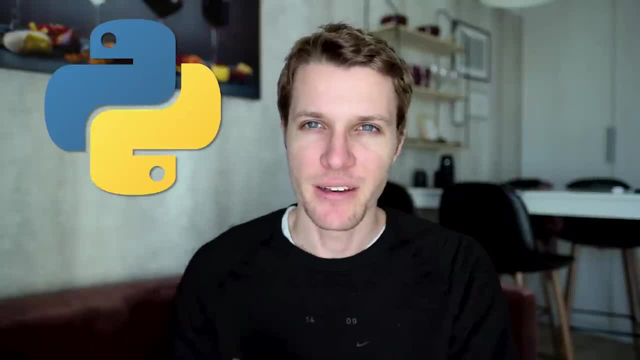 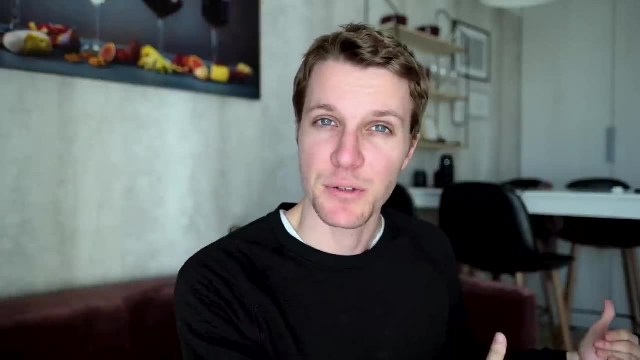 moves from language to language, from c to javascript to python, and it's not because it's covering as many languages as possible, but rather focusing on the logical elements and patterns instead of the specific code samples. Okay, now let's talk about coding, which in some ways, is 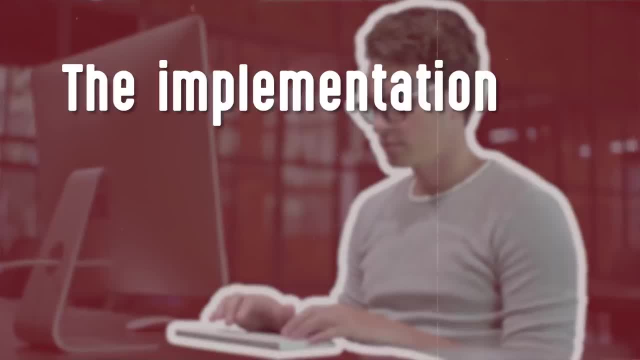 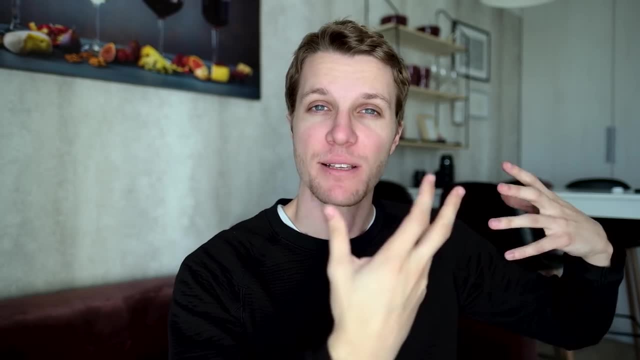 broader and in others more specific. We could call coding the implementation or details of a logical programming solution, But, as we know, that's not necessarily the case, because we can also code in something like html or css. For this reason it's harder to pin down a specific definition of coding. but one thing's: 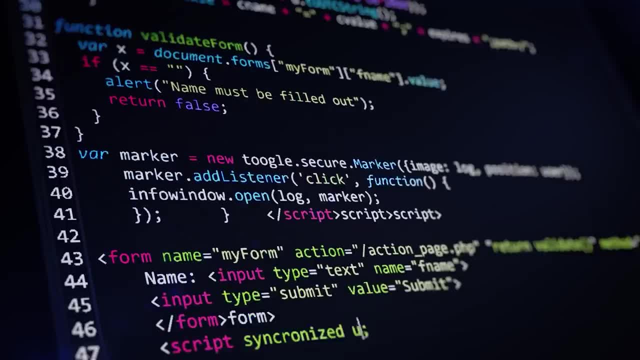 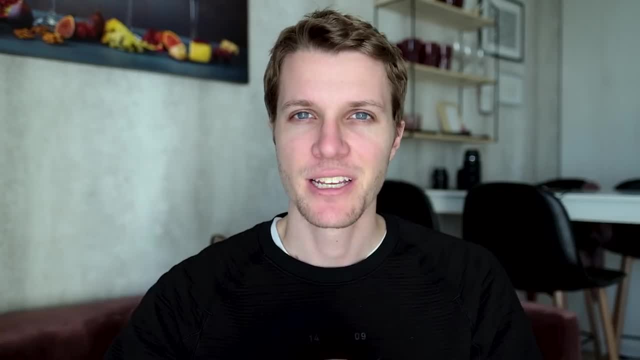 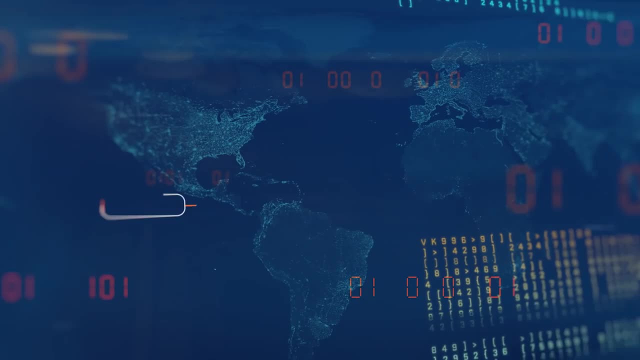 for sure to be a good coder, you have to learn the syntax of different coding languages. In many ways, the logical problem solving of programming is on a higher level of abstraction than coding, which is more focused on technical details. Details like code quality, breaking things into functions and different files, and leveraging code libraries all come into play. 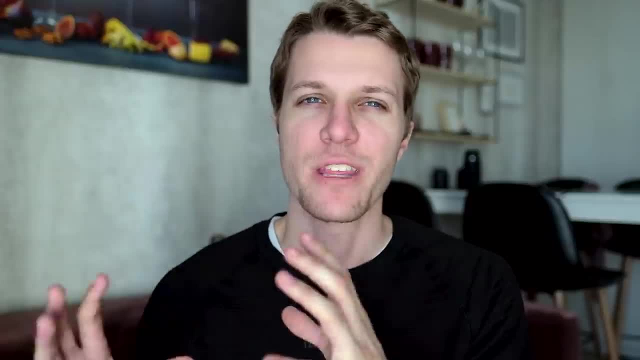 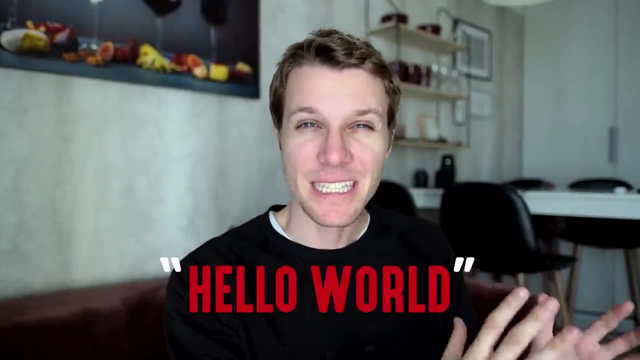 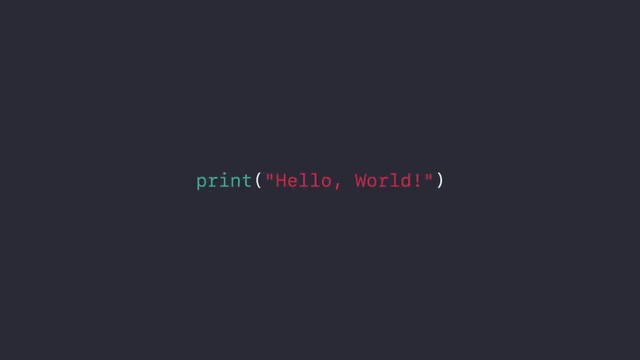 now, interestingly, you can swap out different code solutions for the exact same programming outcome. this is part of the reason the first code we write in any new language is hello world, which is completely the same in programming terms but different in every language in coding terms: javascript, console log, python print and the java one. that is super long. 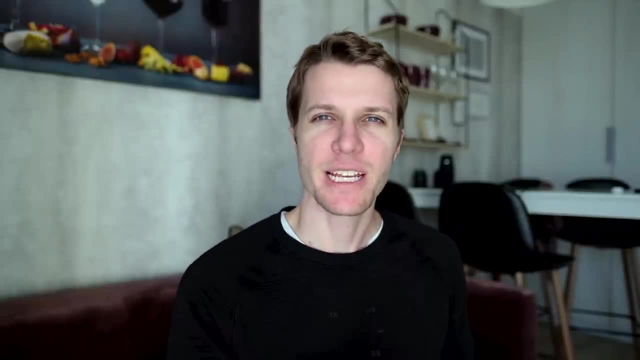 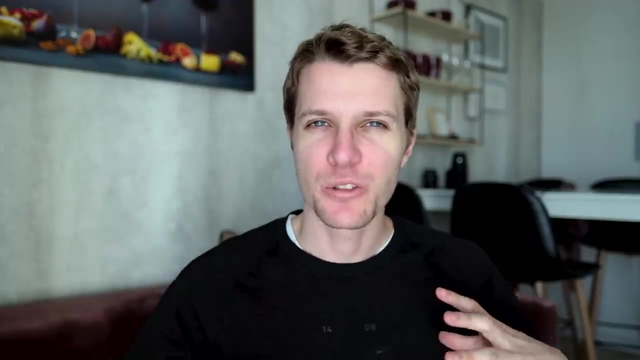 just like everything in java. one important thing to keep in mind is, if you try to explain coding details to non-developers, they will quickly fall asleep. this is where some of the old conflicts between technical and non-technical people on a team emerge- where the developers are. 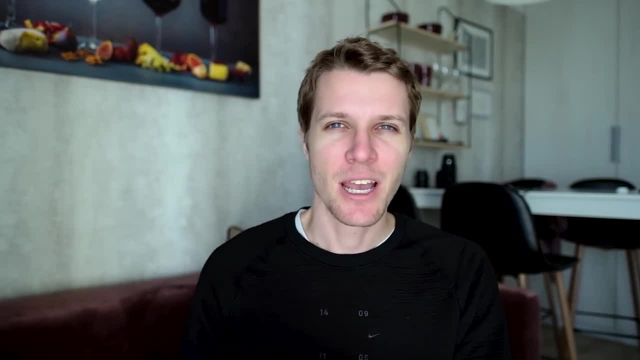 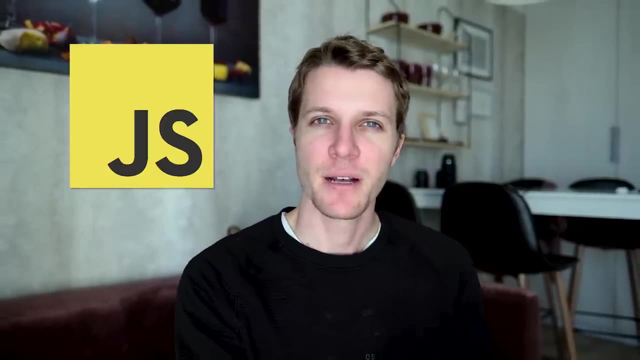 pushing to refactor the code base. the project manager is asking what's the benefit to the end user and met with blank stares. to give a course example for coding, if you see anything like basic javascript, python 101, advanced python- these are very focused on pure coding concepts. in other 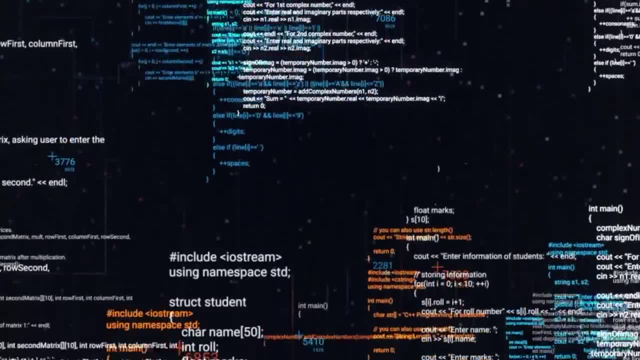 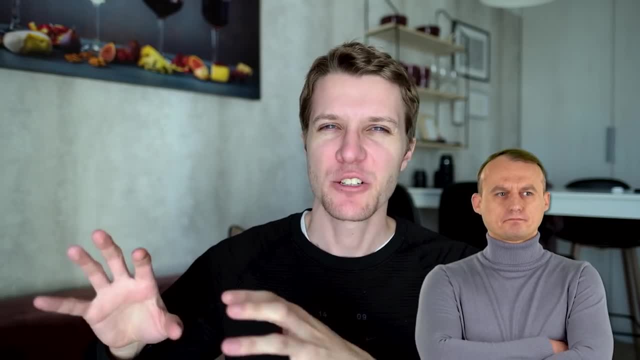 words, the syntax and patterns of a specific language. also be a bit careful. calling someone a coder is a bit slanderous in the developer world. it kind of implies that you're just a cog or a machine and all you're good for is writing code, and also that you're easily replaceable by another. 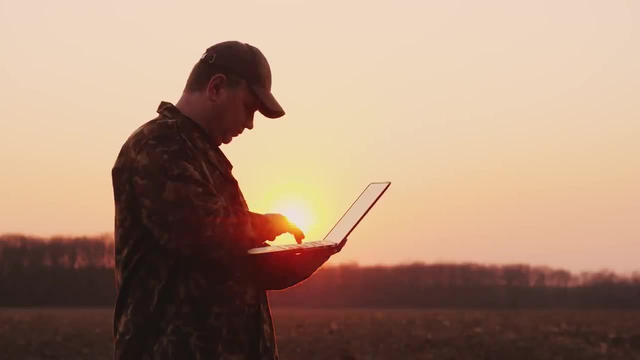 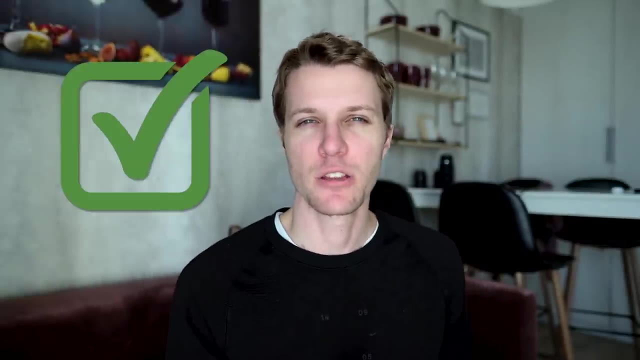 coder, and that person could also be on the other side of the world. so with both these definitions, it's fair to say that once you know programming, coding is really easy. it's why experienced developers can learn new languages so fast. learning programming also helps you build mental. 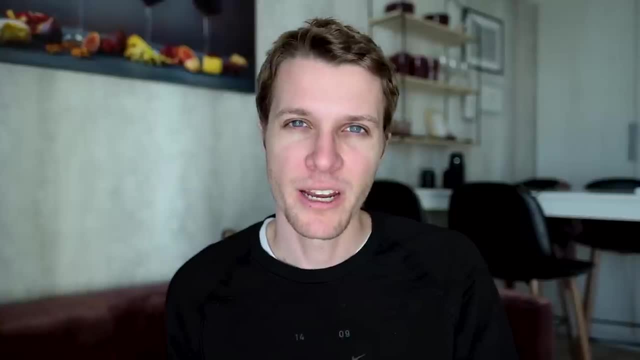 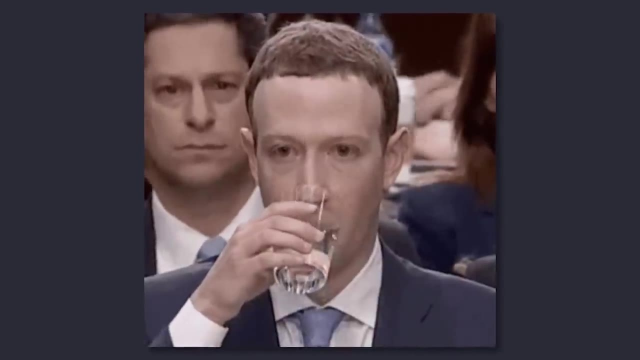 models, and i think it's no coincidence. the world is now run by former programmers- bill gates, jeff brisk, mark zuckerberg- and for this one, let's just leave their reputations out of it. so you will hear a lot of people say: focus on programming when you're starting out, don't worry about coding. 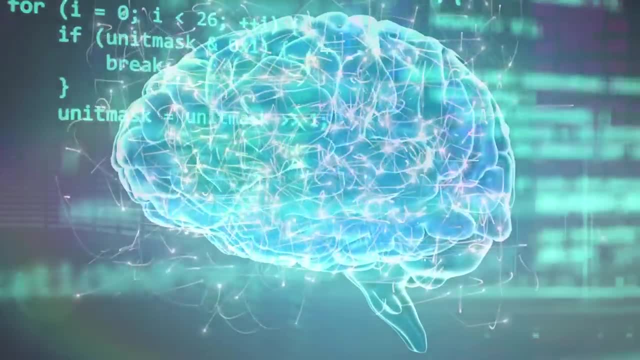 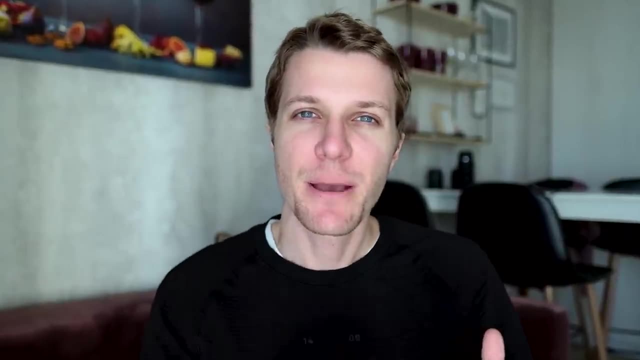 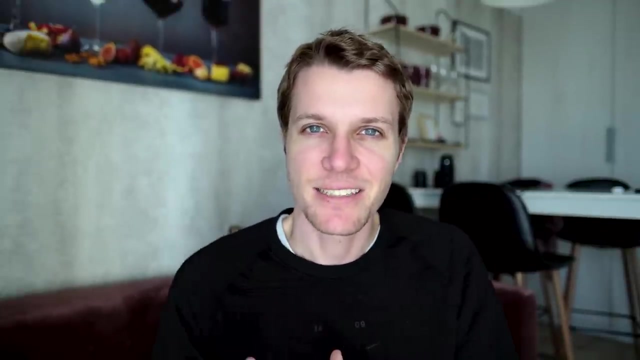 language and people think this gives them permission to go learn five different languages just because they're not focused on language. but the truth is, the faster you can master a single language, the sooner you can get beyond just the coding step and you can only focus on the programming because you're not constantly learning a new syntax anyway. just a bonus here. 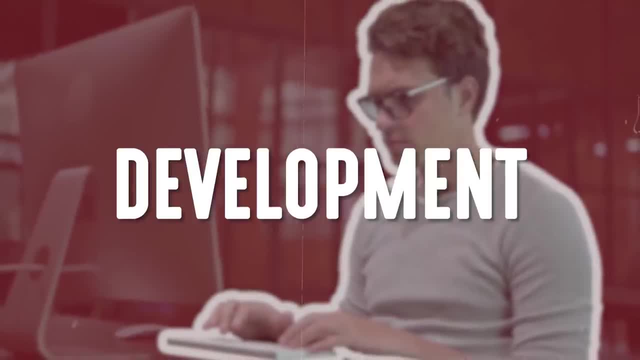 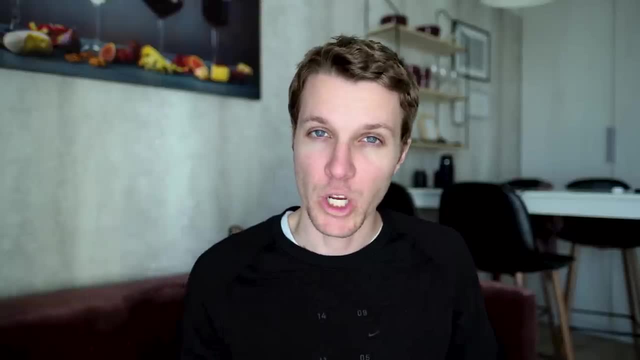 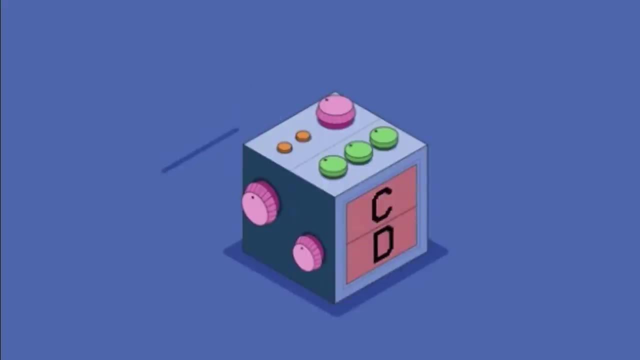 at the end. let's compare both of these to. development is more focused on the solution outcome or business need, and development solutions can involve much, much more than programming or coding. now, while we do see coding jobs automated more and more by better tooling, code generators and even machine learning, 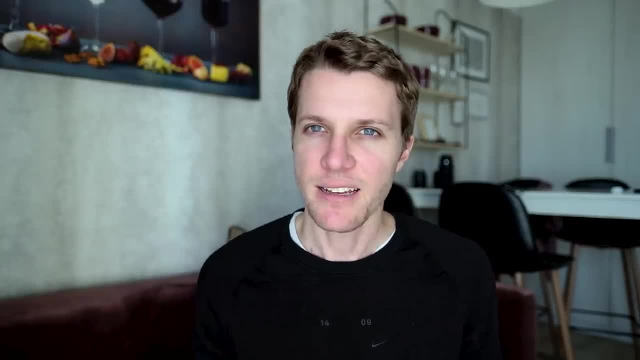 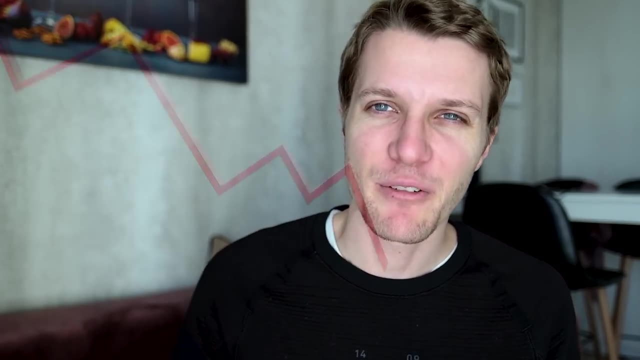 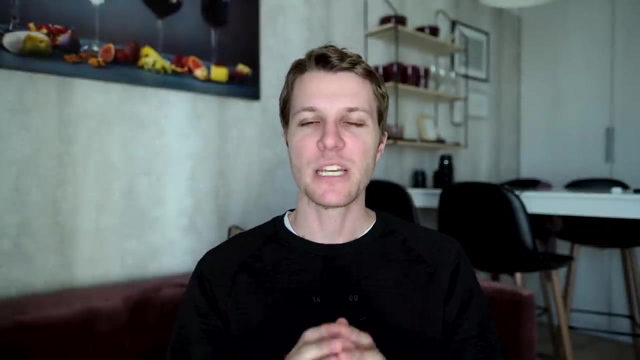 algorithms, the principles of programming are here to stay and we could see the number of jobs requiring pure coding drop. even if you move beyond the job of being a programmer and want to become the next elon musk, it can still help you a lot anyway. i hope this video illuminates some of the key